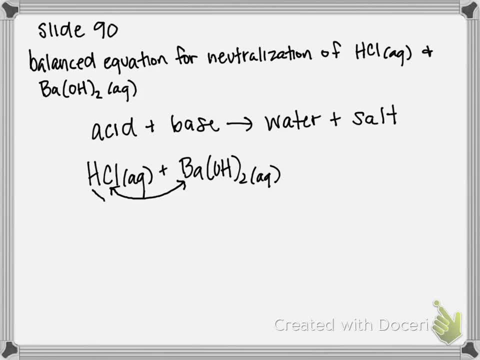 and that means the positive ion of our acid is going to go with the negative ion of our base. So currently ignore the subscript On the hydroxide when H and OH combine H-O-H. what's another way to write that? 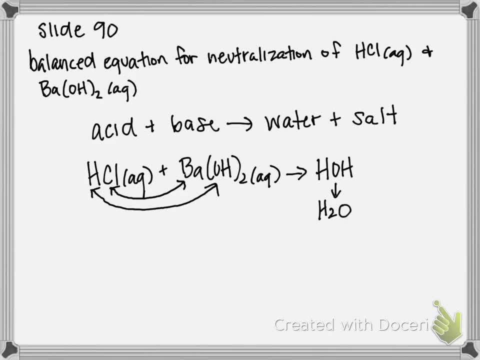 H2O And to B-A and C-L are going to combine. barium has a two plus charge, Chlorine has a minus one charge. So therefore my formula is going to be B-A- C-L-2, because I need two chlorines to balance that one barium. 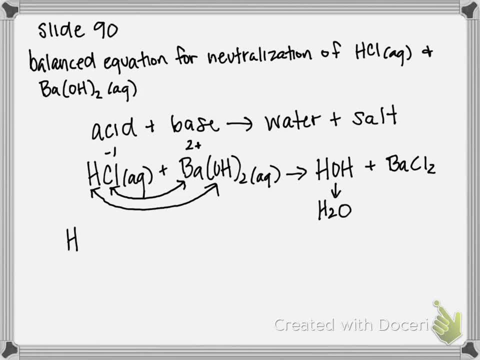 So I can write HCl, which is aqueous, plus barium hydroxide, which is also aqueous form- I'll move that over a bit- H2O, which is a liquid, and barium chloride, which is also aqueous. 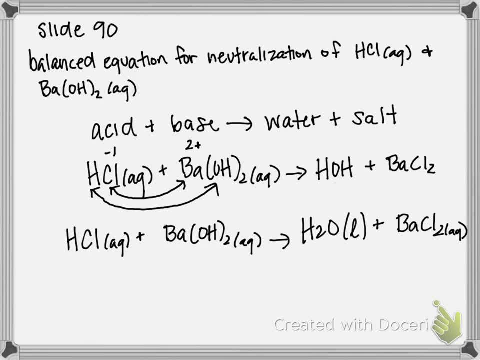 So now the last thing we need to do is make sure that this equation is balanced And- spoiler alert, it's not balanced, so we're going to have to balance it. So I'm going to look at my chlorides first. I have two chlorides over here, one over here, so that means I need two in front of my H. 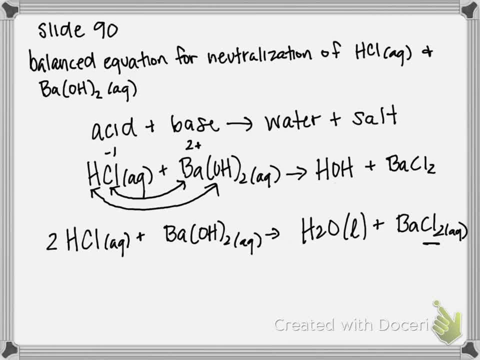 And now I'm going to count up barium. Both have one Hydrogen. we have two HCls and two hydrogens from the hydroxide on the reactant side, So that's a total of four. We only have two on the product side. 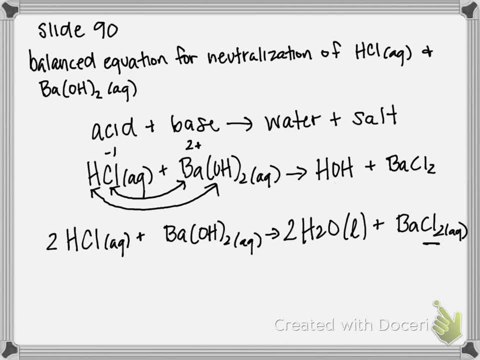 So that means I'm going to put a two in front of my H2O. So now, if I count up two hydrogens and two hydrogens, so we got four H's on this. two from here, two from here, We got.